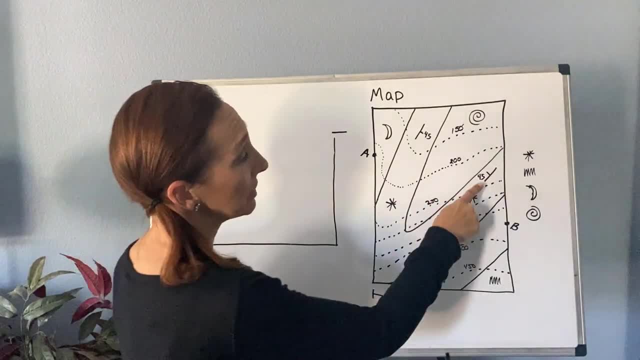 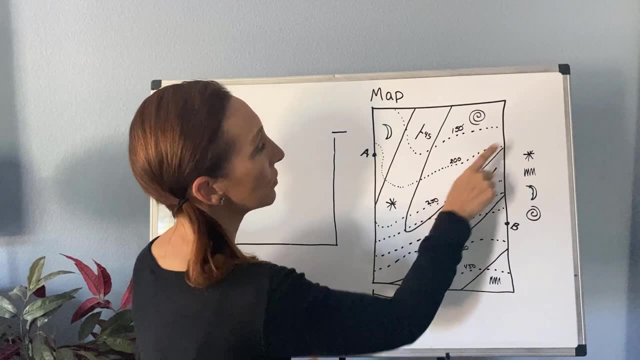 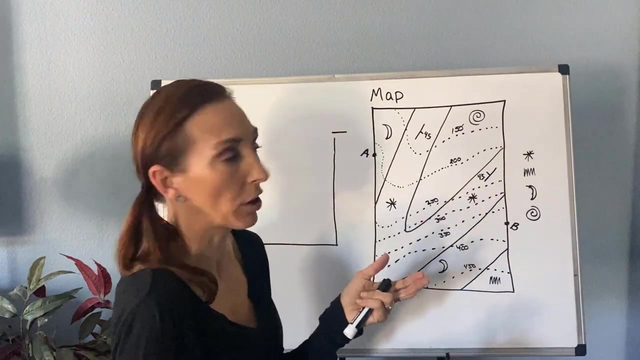 assumption. We also see a couple other things. We see a couple strike and dip symbols here. So this asterisked unit is striking kind of northeast, southwest in both locations And then the dip is going toward the center of whatever the structure is at a 45 degree. 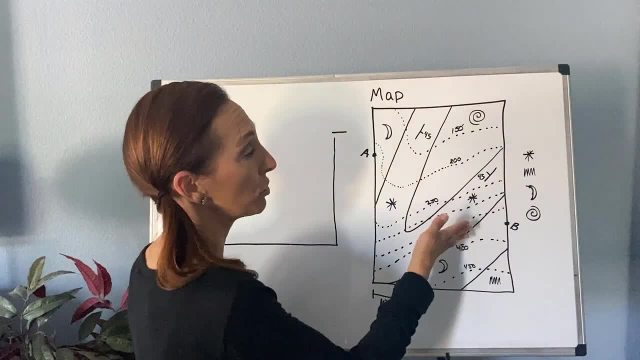 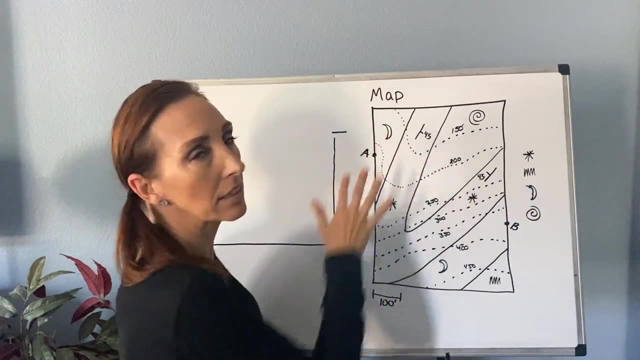 angle And the directions would probably say something. like you know, assume all the beds in the lower right corner or the southeast corner are dipping, just like the asterisk one there, and then the same thing about the northwest corner. So we're going to make that assumption. 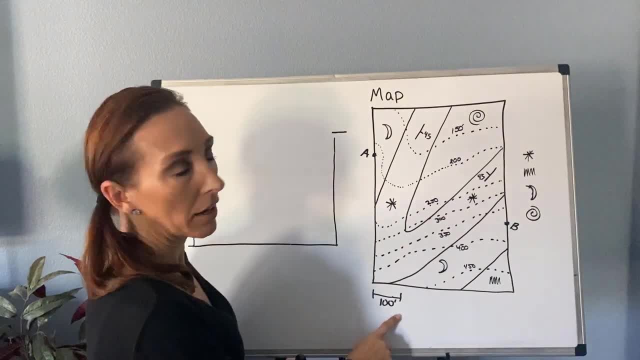 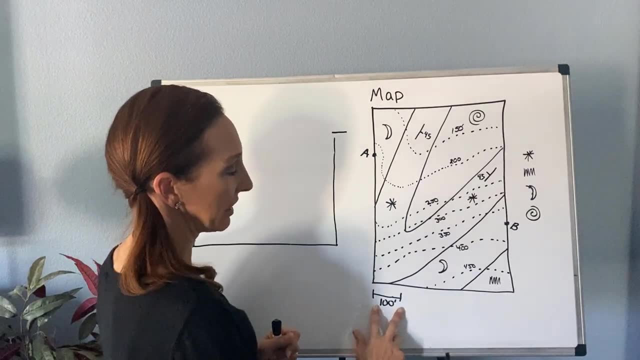 as well. I also see that I've got a little scale bar at the bottom, So this isn't like a true map, it's just something easy for me to illustrate with. but we're going to say that this amount here is going to be 100 feet. So across the map, 100 feet is represented by each of these kind of 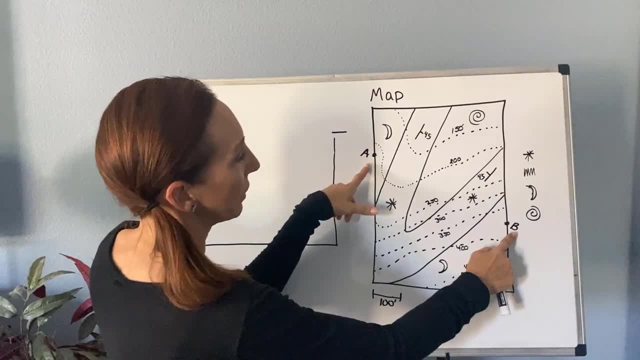 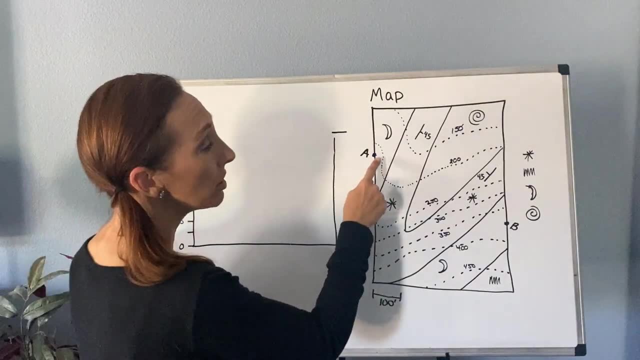 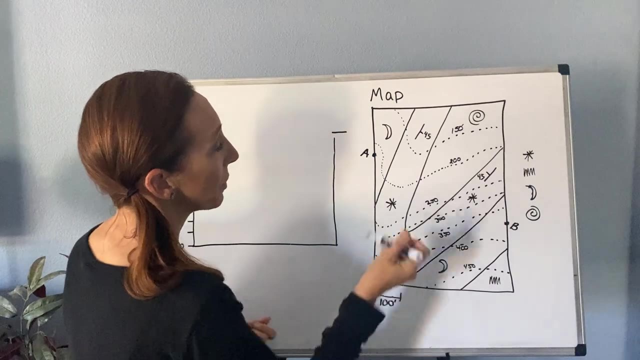 bars, And then the final thing that I see is this point: A and B are marked on there, And so what will happen is we'll say: let's create a geologic cross section with a topographic profile across from A to B. So what you're going to want to do, typically, is make a line that traces across there. 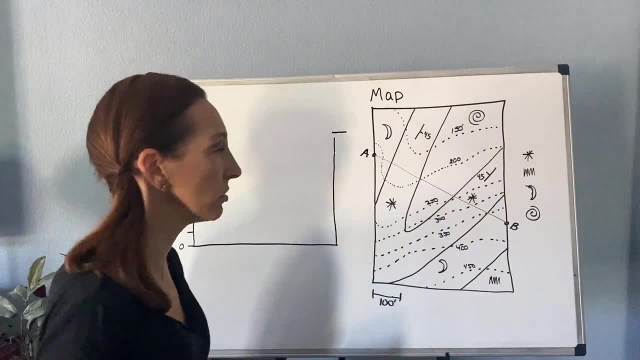 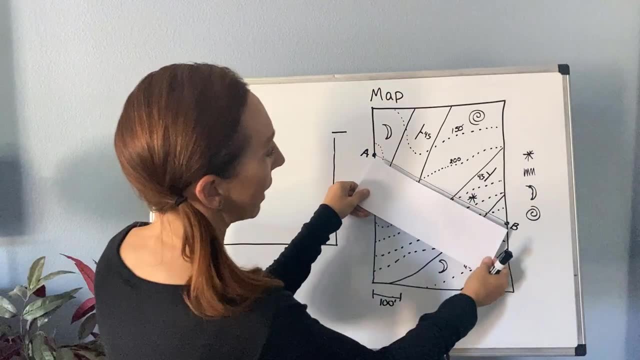 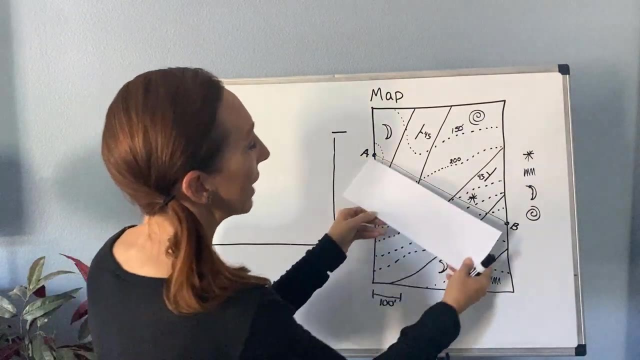 with the ruler and you know some kind of pencil, And then we're going to get a strip of paper. So I have my strip of paper and I've made it exactly the length of that there, But yours can go beyond that. I'm just doing it because of the dry erase marker. And if it is beyond that, what? 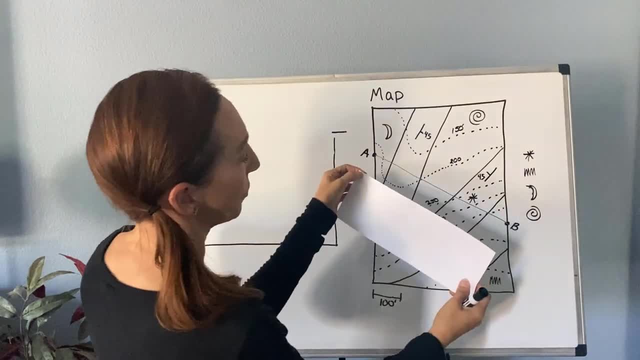 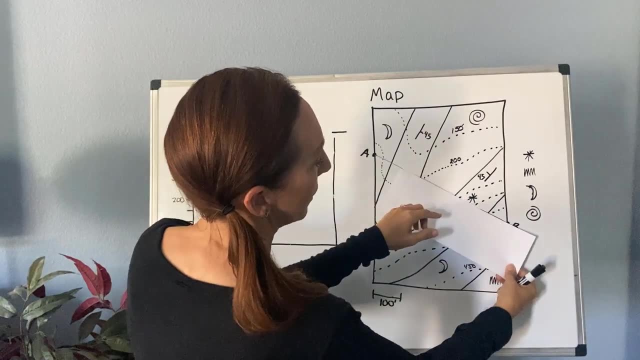 you would. first thing you want to do is you want to indicate that where the A falls and where the B falls- So let's say that your paper was longer- you would make a little tick mark here and put A, and then, if the paper went beyond there, you would make a tick mark there and put B. 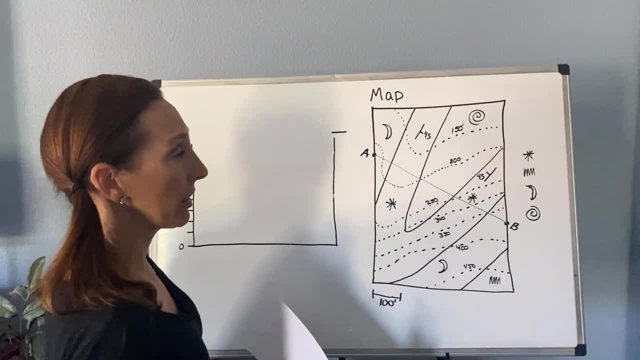 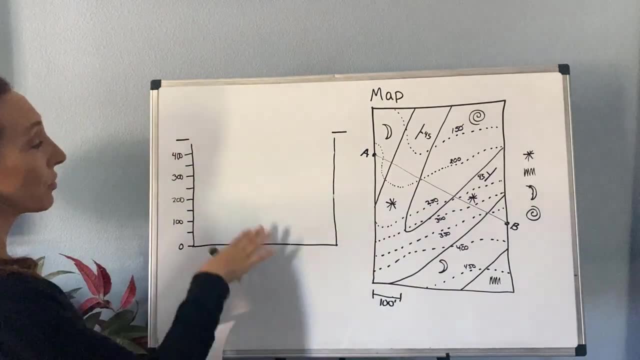 So that every time you line up your paper it's going to be lined up in the exact same spot. Okay, so now I have a piece of paper that's the width of this section that I'm going to be drawing And you'll notice over here I have this, uh. 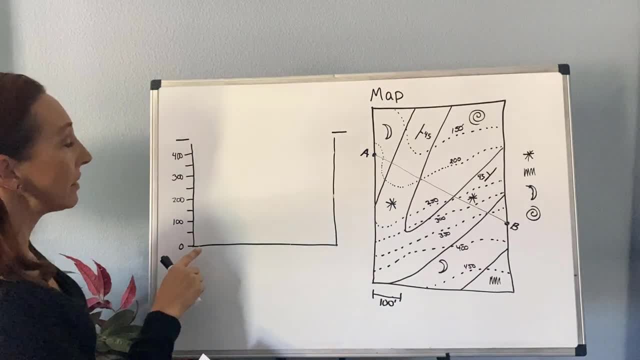 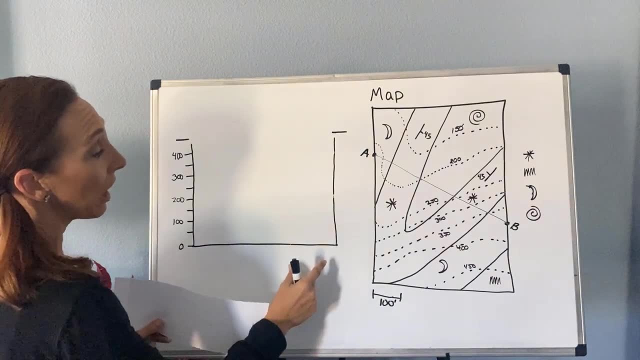 kind of template already drawn and i pre-filled it out a bit and you'll notice it's the same length as that line. so that's going to be really important to do that and in this case, because of the scale i've chosen, 100 feet is going to be represented across the bottom here. so it's about. 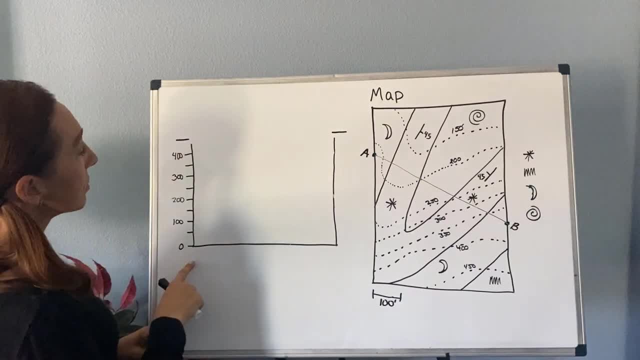 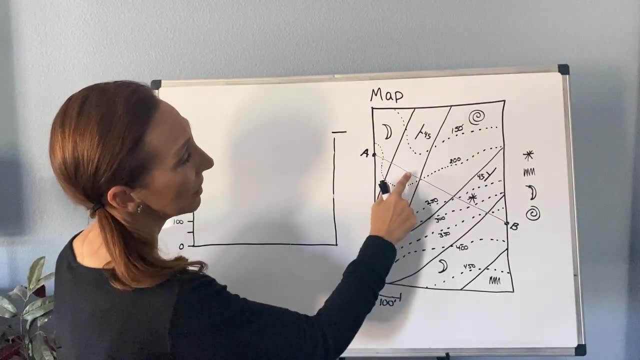 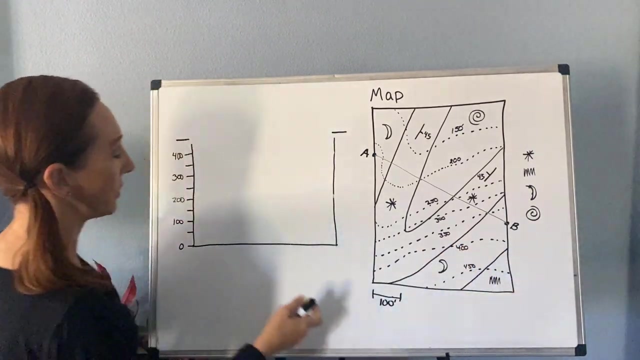 500 feet or so across that line, um, and then we're also going to see that my vertical axis i've already went ahead and labeled with the appropriate values. so i noticed that i had values from 150 to 450. um, i'm not my b line or my line doesn't cross anywhere near the 450. so i started at zero and 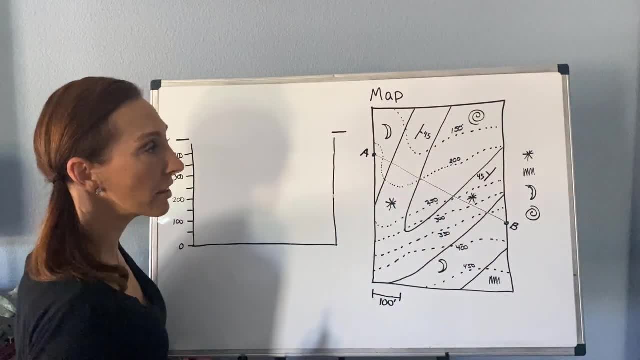 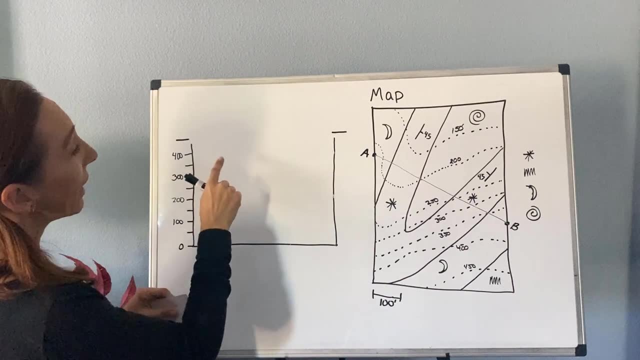 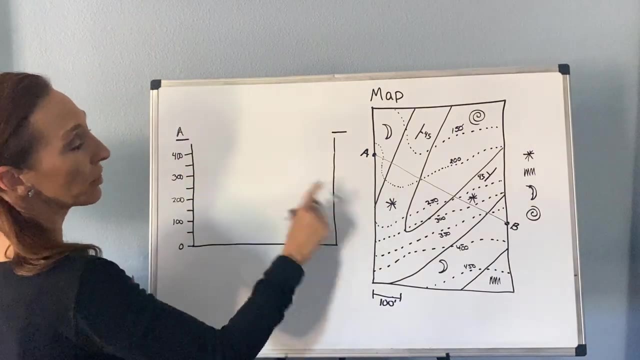 went up and ended up at 400. that's going to catch all the contours that i need to that actually cross this line. that'll make more sense in a second. all right, so, um, i also want to designate that the left hand side of this is the a point and the right hand side is going to be the b point. 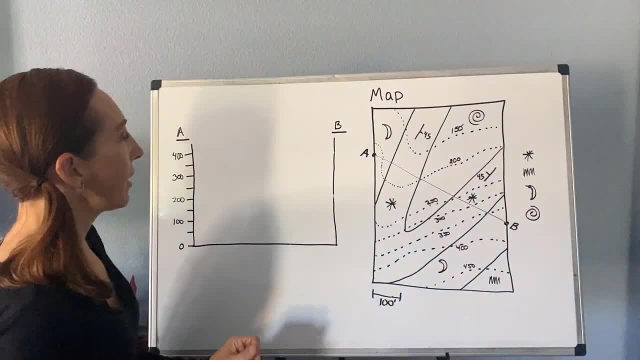 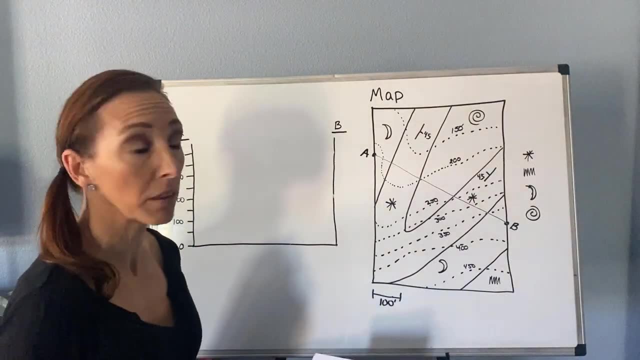 because technically you could do it backwards, but that would be a little bit weird. um, so now we're going to go ahead and get started. so i'm going to first start to mess with my- um, the actual topographic profiles. that's going to be the contour lines, that's going to be the 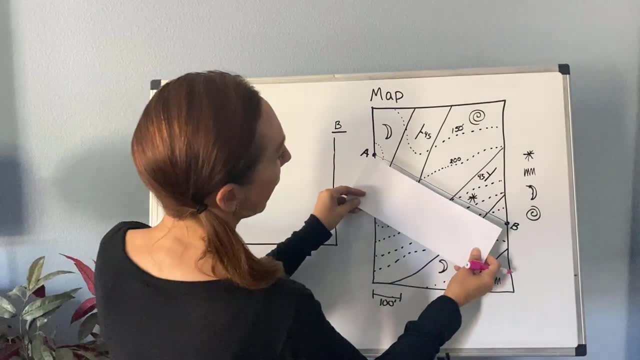 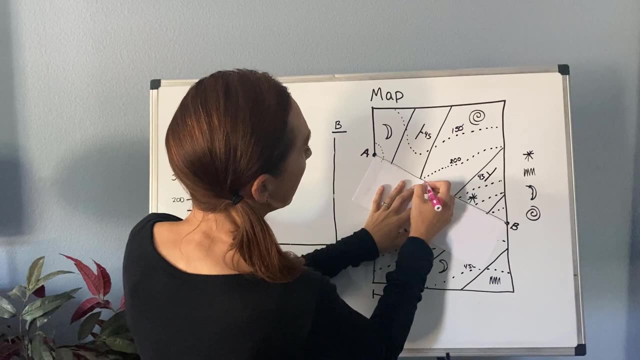 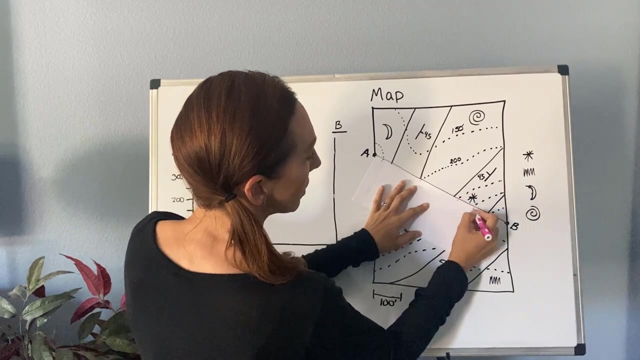 easiest thing typically to start with, okay, so i'm going to put my paper across here and hopefully not erase too many things in the process, and i'm going to make little tick mark there, anywhere that the contour crosses my line. i want to make a mark, all right, so i make this a little bit bigger, probably. 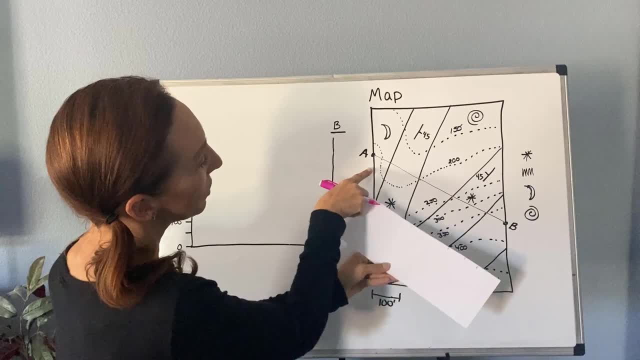 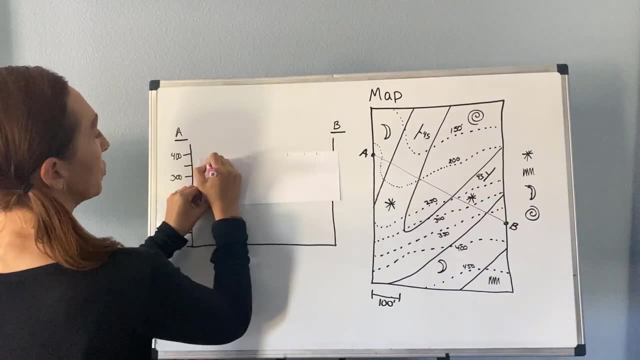 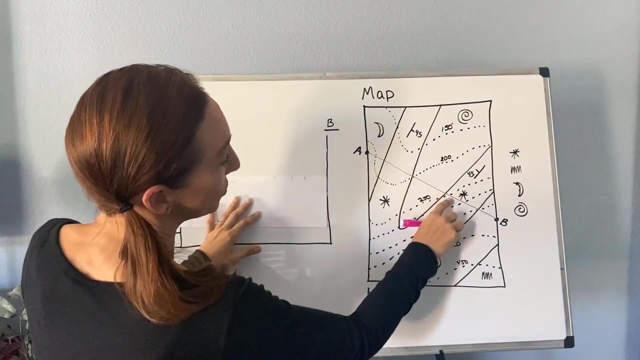 but now i have these marks here and i'm going to notice that these first two are the 200 foot. it crosses twice. so on mine i would label 200 and 200 and then i would notice that the next one i crossed was this: 250, then a 300, then a 350, so i would label that 250. 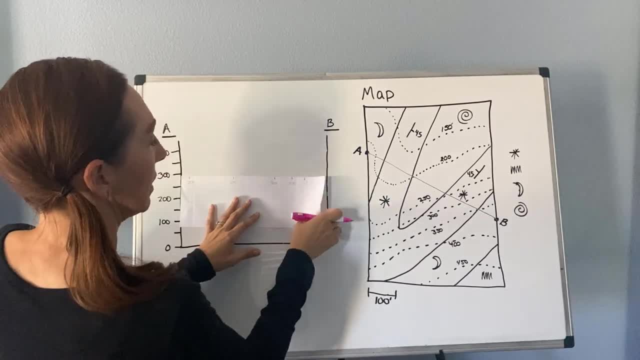 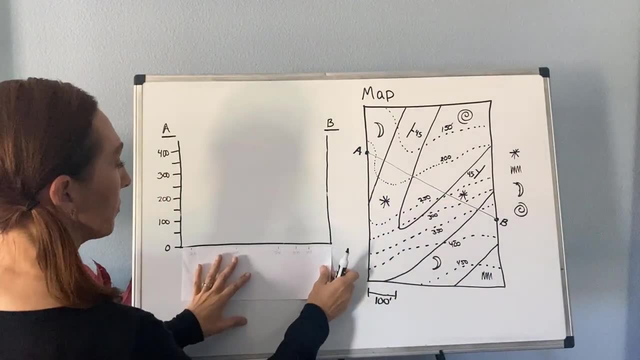 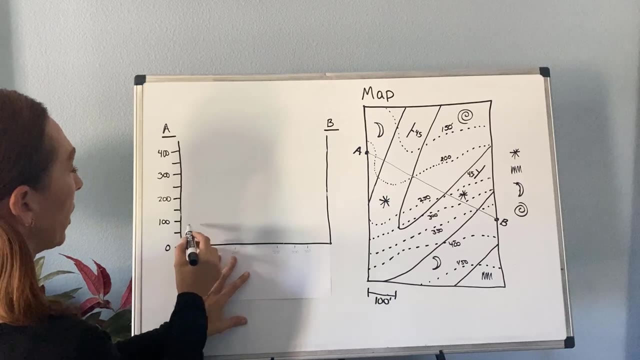 300 and 350.. okay, so you'll have to trust me. that's what that says there. okay, so now i'm going to take my piece of paper and i'm going to put it across the bottom of my cross section and i'm going to say, okay, there's a 200 foot contour mark here, so i'm going to go. 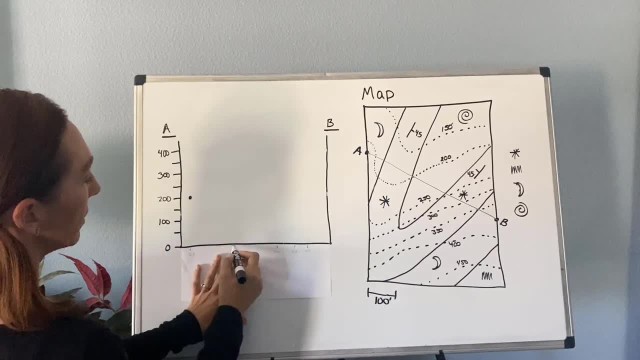 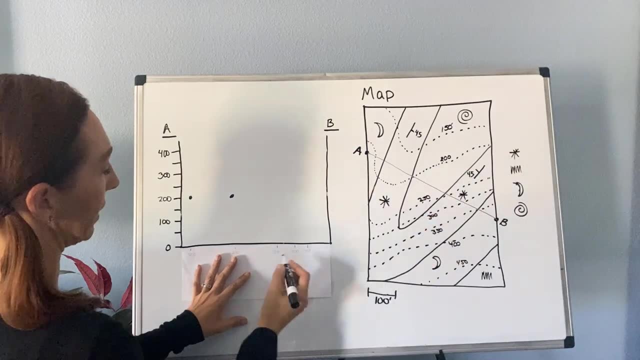 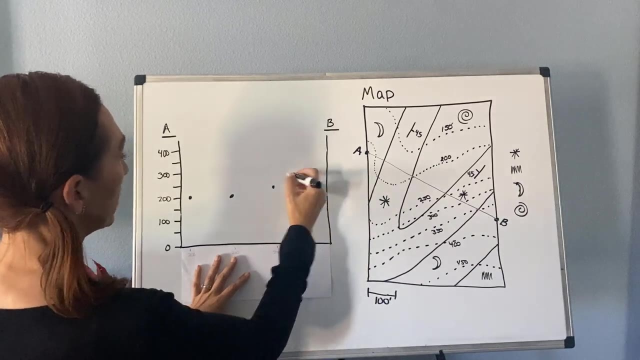 up to 200 and make a dot. and then same thing here at 200, and this again is the elevation, the topographic profile, so the shape of the land surface. I'm going to go above the 250, make a dot there, go above the 300, make sure it lines up with my. 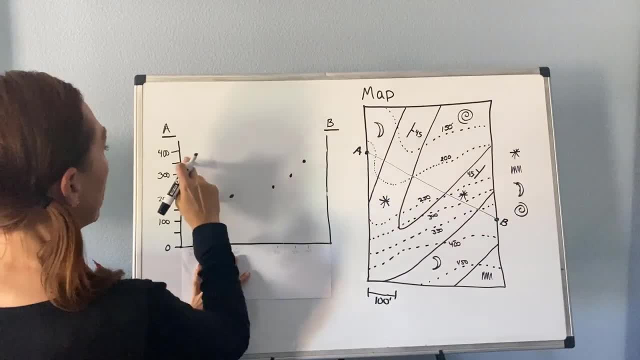 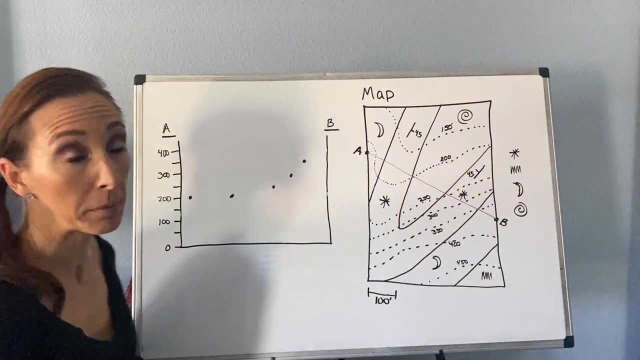 300 there and then 350, make sure it lines up with my 350 there. So these are the elevations as I traverse from A to B. So I need to connect my line. So what I'm going to notice is: I don't. 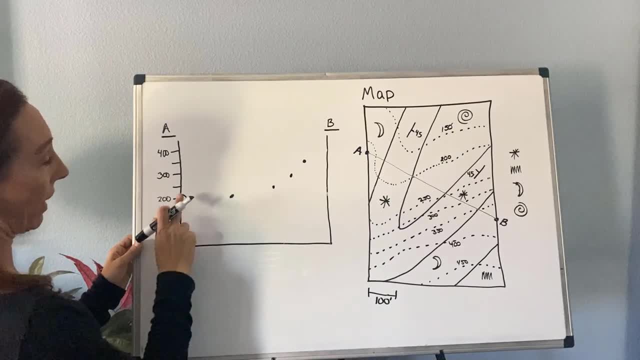 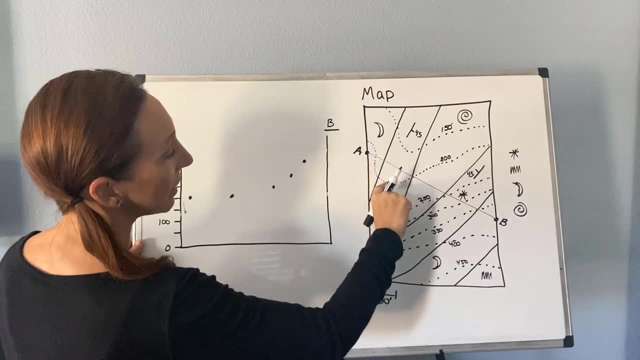 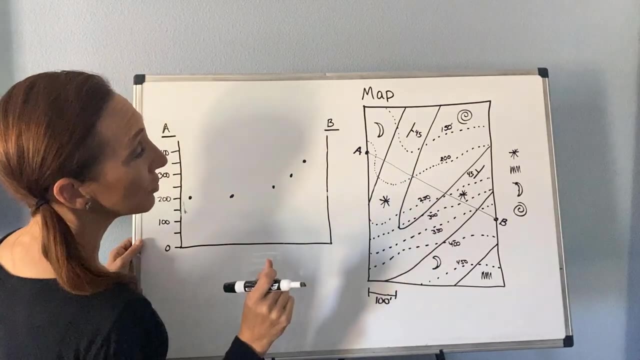 need to figure out: is this coming up like this or down like that? right? And so we can look at it here. If I go between that first contour and the point A, I would notice that I'm increasing in my contour value, So 200 to 250.. So this has to be above 200. So it would be coming down and I don't. 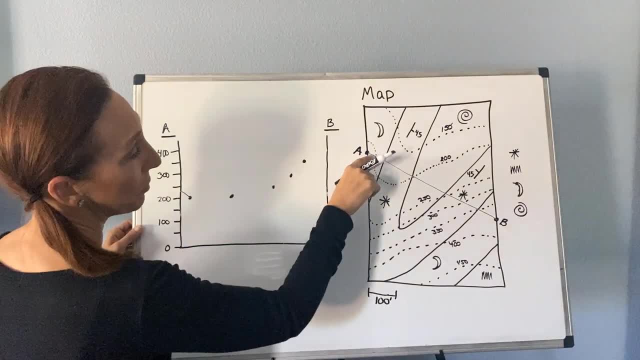 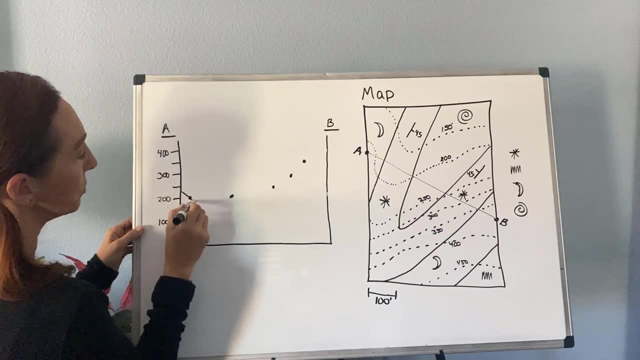 want to get too close to the three or the 250, because then it would have picked up another contour there. So I'm going to start at between the 200 and 250, come down, and I'm going to swoop down and then come back up And again I don't want to get. 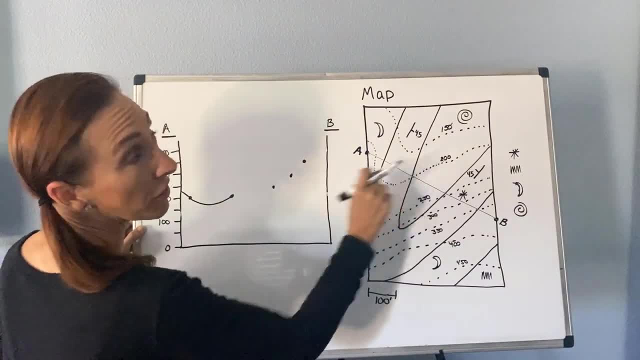 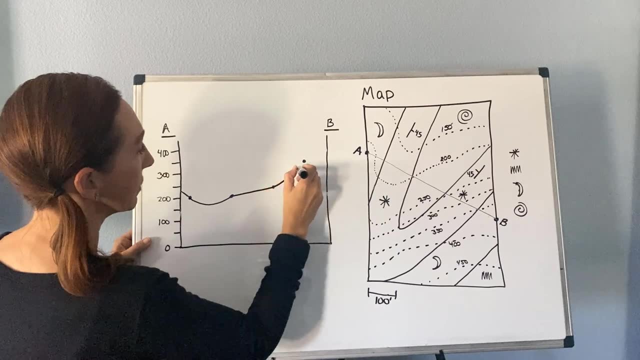 too close to the three or the 250, because then it would have picked up another contour there. If I get too low here, I would have picked up another contour there. So I don't want to get into that 150 range And I'm going to come here and connect the rest of these Same thing. I don't 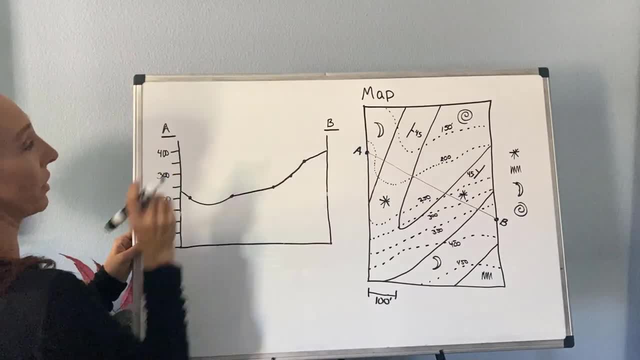 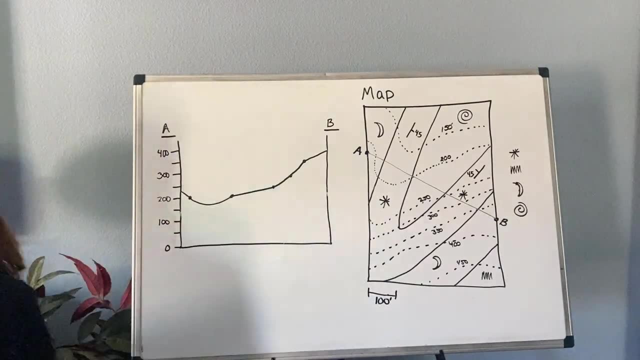 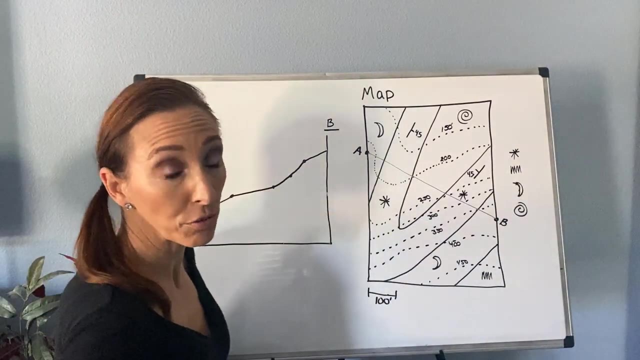 want to go too high, because I didn't pick up that 400 foot contour interval there. So now this is my land surface, So that's successful. And so now what we want to do is we want to come back here and do the same thing, but with the actual. 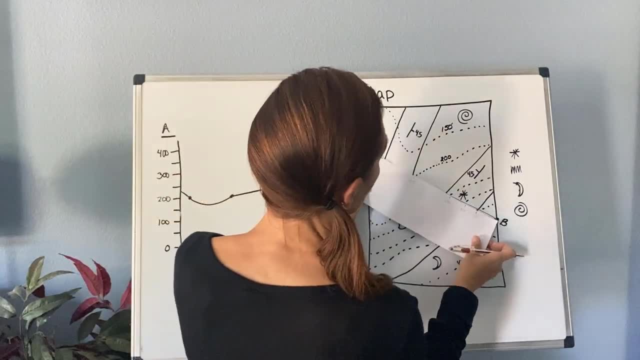 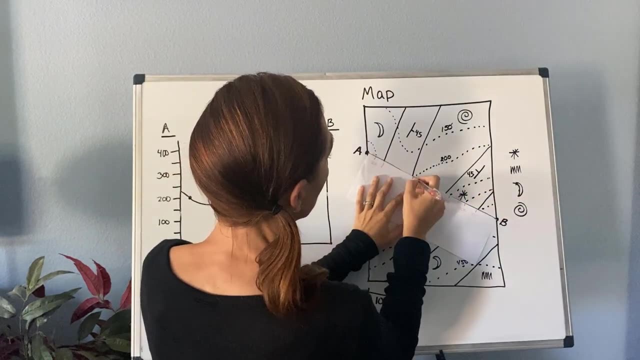 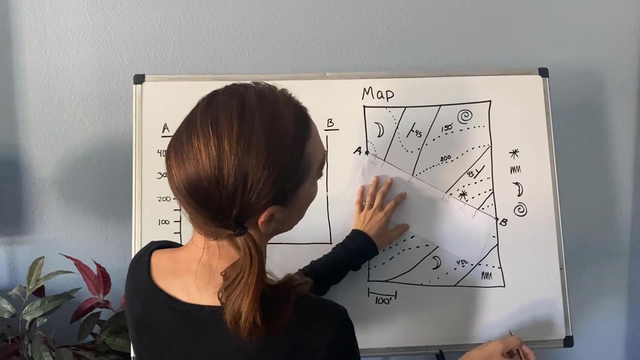 geologic units. So if I come and put my paper across here, what I'm going to notice is that my geologic units- I'm going to use a red pen- come here, here, here and here. And if I notate, 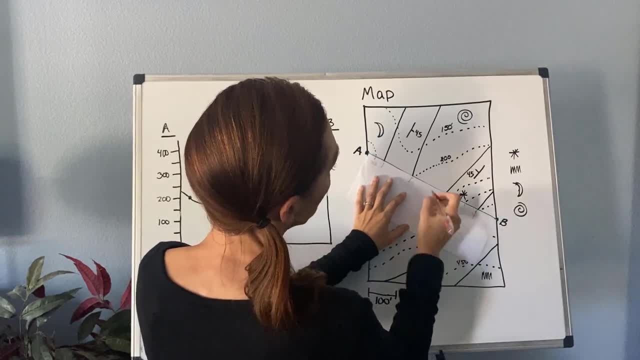 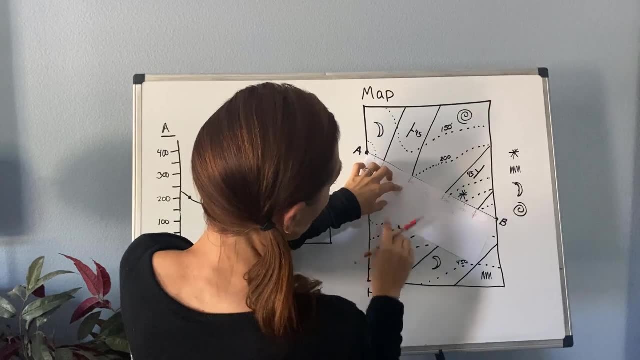 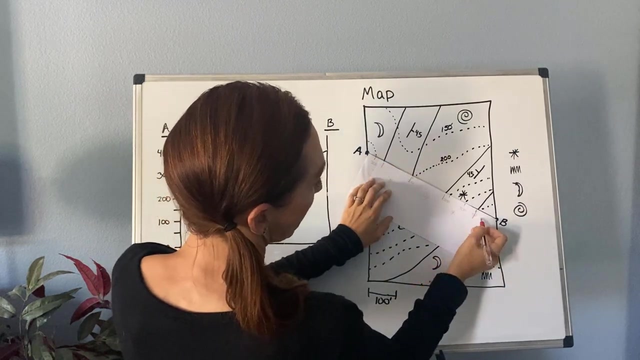 what those are between these two lines. it was an asterisk Between these two lines. I have my spiral Between these two lines. I'd have to look down, but I would find out that it's an asterisk. And then between these two lines it's a moon, And so the only other one I have over 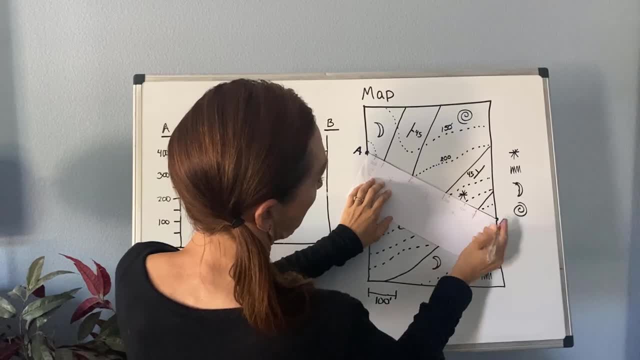 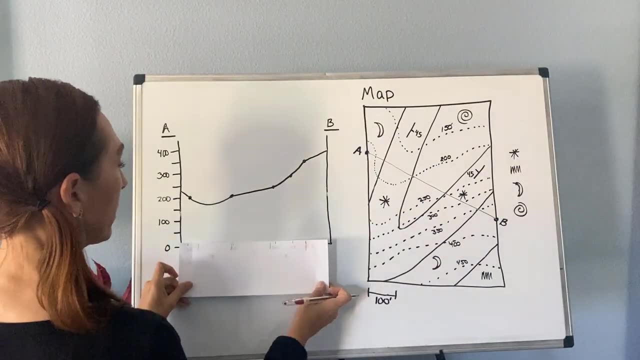 here. this is a moon as well, So I did that backwards, but that's okay, All right, So now I can put these onto my map here, So I'm going to do the same thing And this is easier to maybe slide. 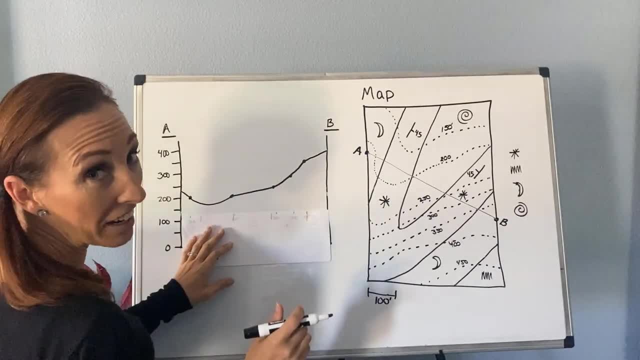 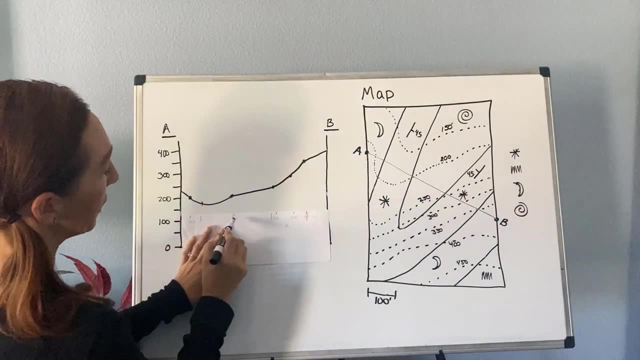 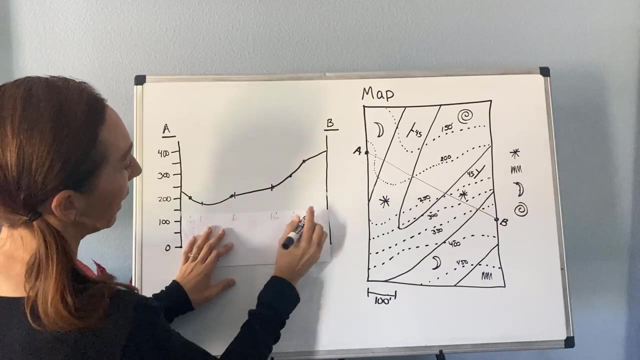 it up a little bit. Okay, We're ready to make our marks. So I noticed that my first bed intersected here on the surface, My next one intersected here on the surface, My next one intersected here on the surface And my last one, if I go straight up, intersected here. 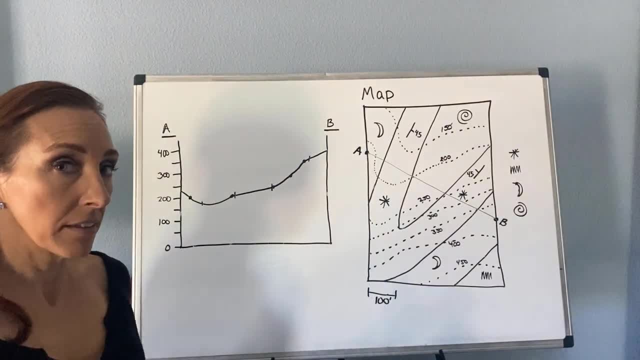 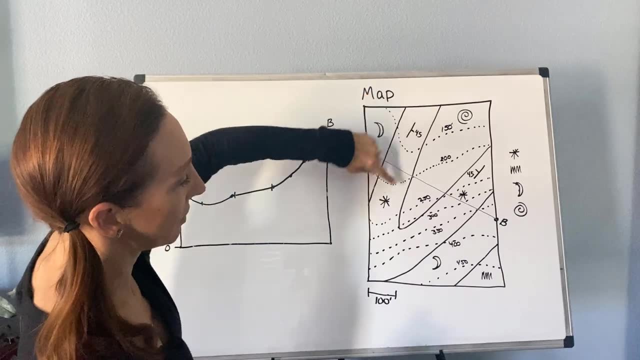 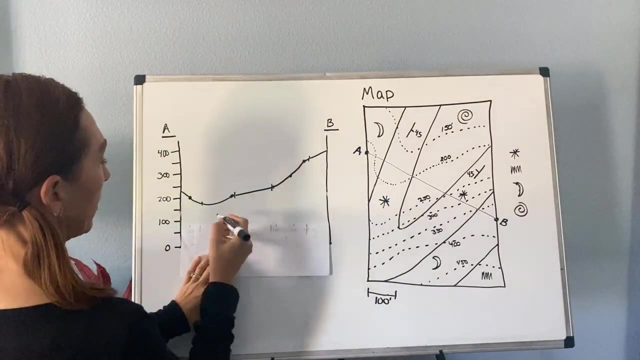 So now I have to determine what direction the beds were tilted, or if they were vertical or horizontal, or whatever the case might be, And so, of course, my strike and dip indicates that this asterisk bed which, if I look, I should have added that on there. So this is going to be my 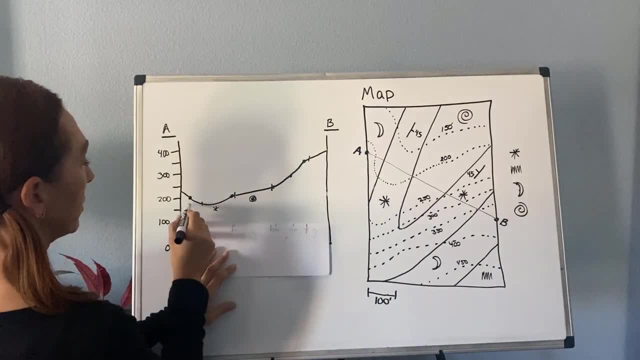 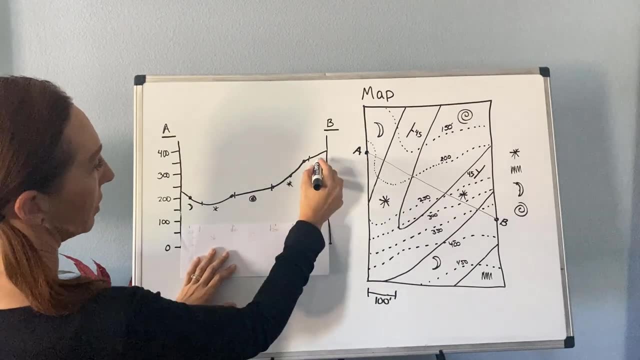 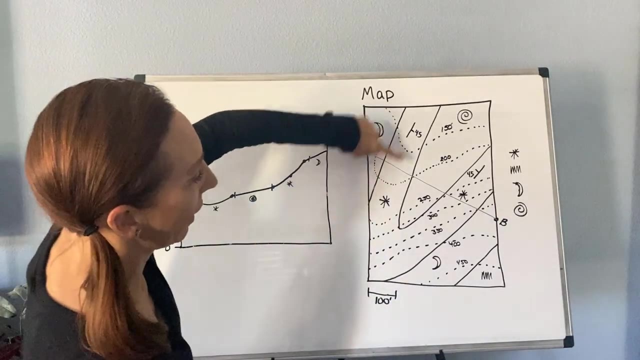 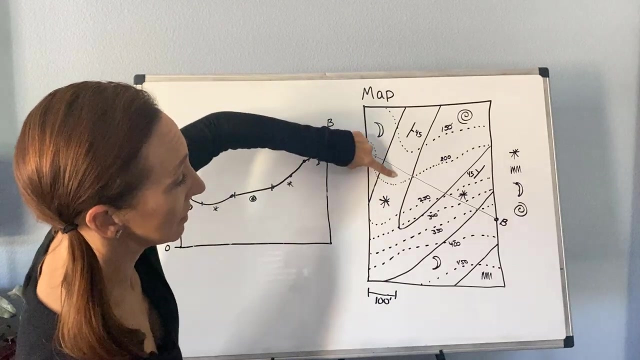 asterisk unit. this is going to be my spiral unit. here's my little crescent banana unit. here is my asterisk unit, and then here's my little moon um banana unit. okay, so if I look back over here I know that my asterisks were striking actually, uh, perpendicular to this line. 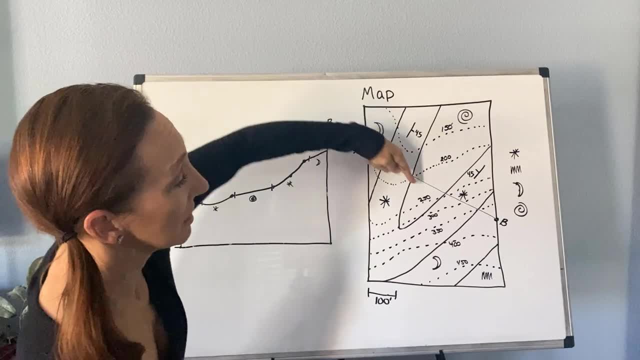 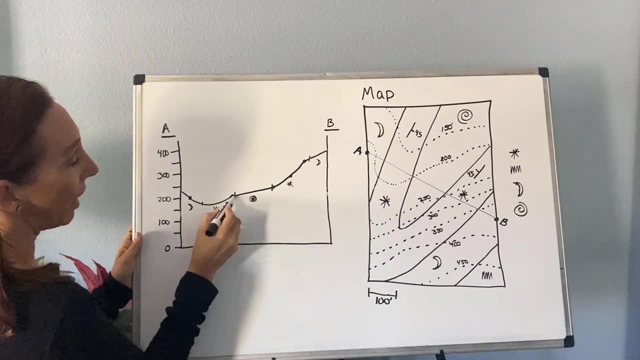 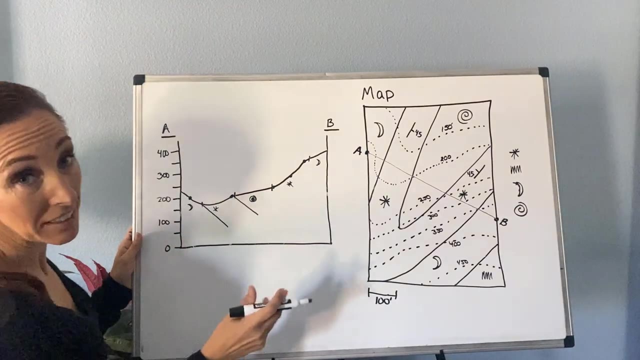 here, which is good. so it crosses right through it and it's dipping toward the center or to the right there, and so what I would want to do- and it's at 45 degrees- here's my asterisk unit- I would dip about 45 degrees and come down and do something like that. I'm not going to go too far because I don't. 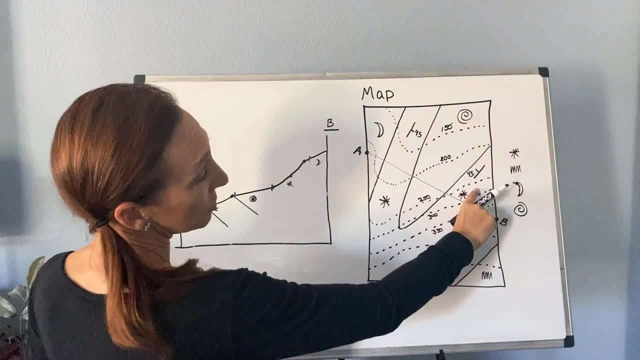 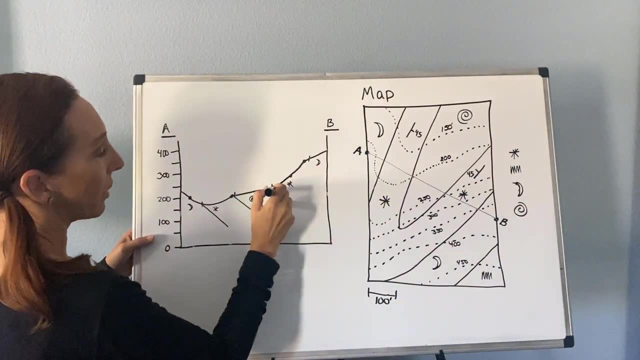 know how far that goes, because I know that my other asterisk unit on the right hand side, so this one here- is dipping the other direction, so in toward the center. so I would do the same thing here, 45 degrees, and then I do my oops. 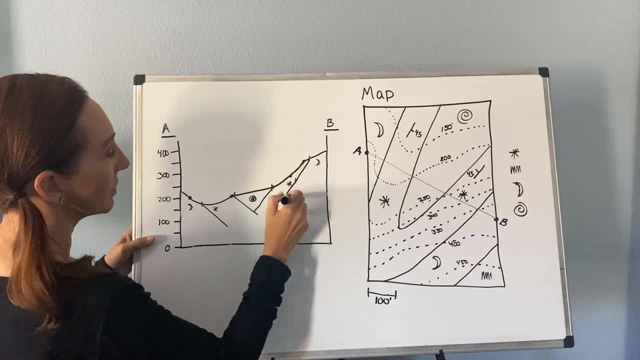 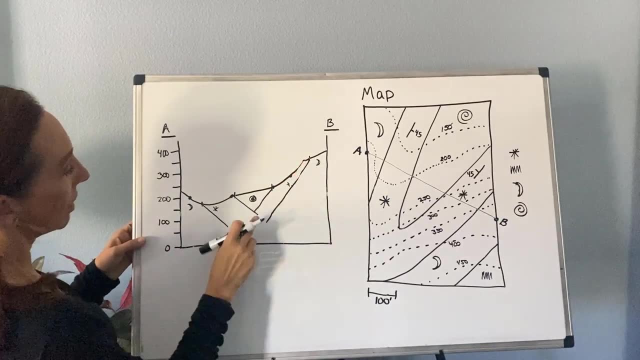 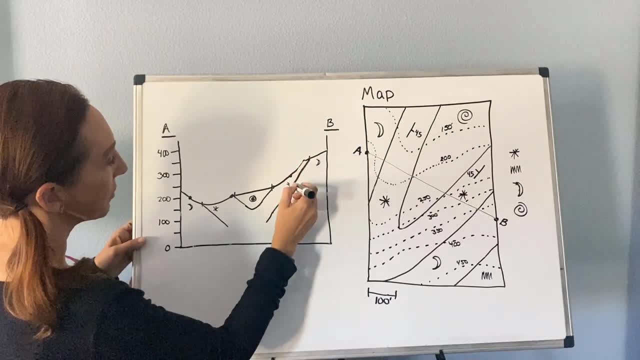 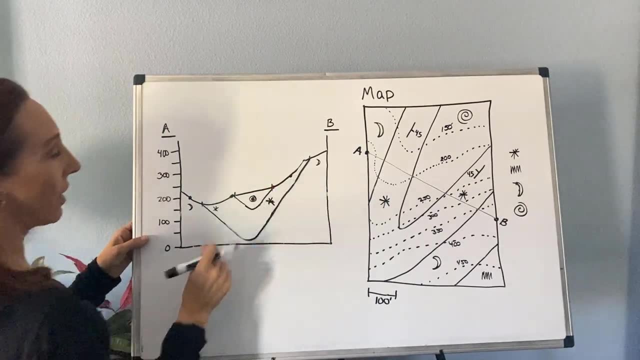 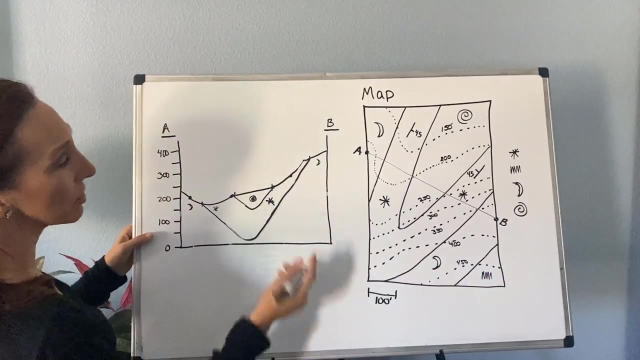 smooth those out a little bit. this one would come down and maybe swoop in, something like that. and so here's my asterisk unit, um, and then my little spirely unit, and then I have my crescent moon, and of course we have our little squiggly down here. so you would assume that the moon unit doesn't go. 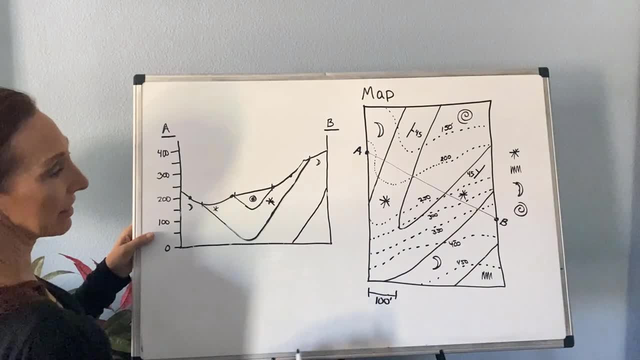 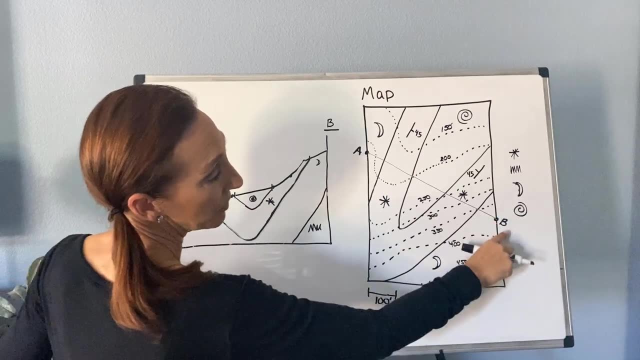 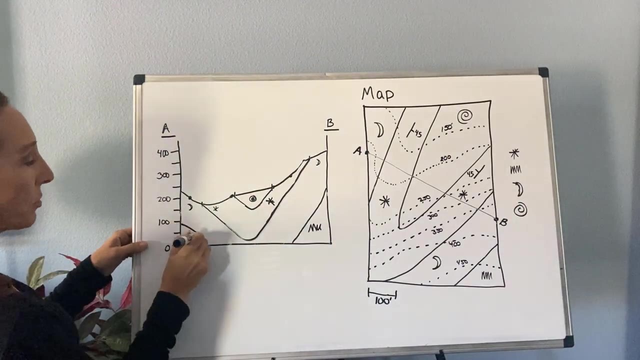 forever. so I'd probably just guess right now and put a line there and then do my little squiggle right, because the moon or the squiggle doesn't get to that um a b line, we'd have to extend our map further to pick up where that would intersect. that okay so, and then I would probably assume 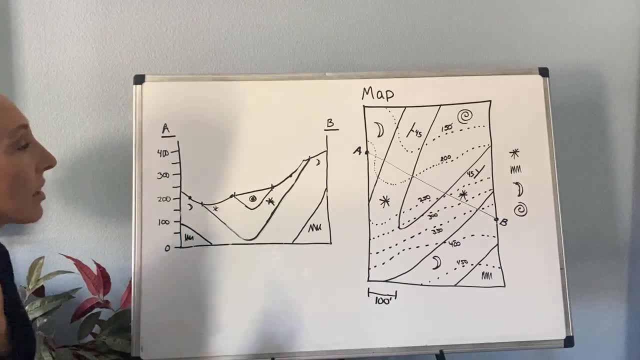 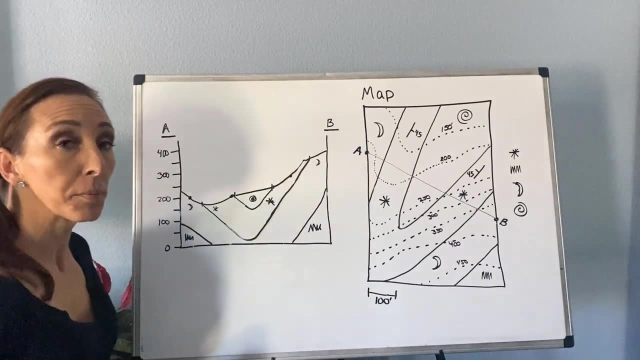 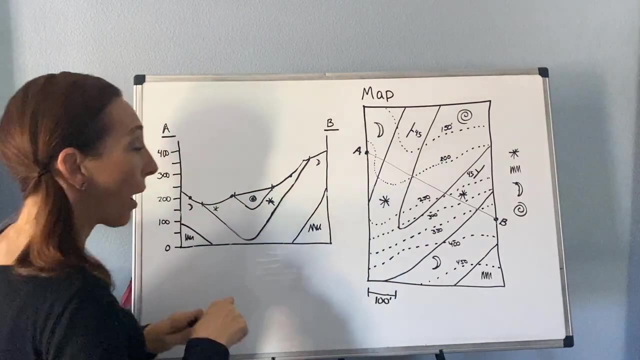 there's another one down here and do my little squiggle there. so now I have my geologic map. I can see that I've actually got this fold in here and if I wanted to, I could put these in order. so we know that if we were to flatten our fold out and go from the bottom up, um, if we went oldest- 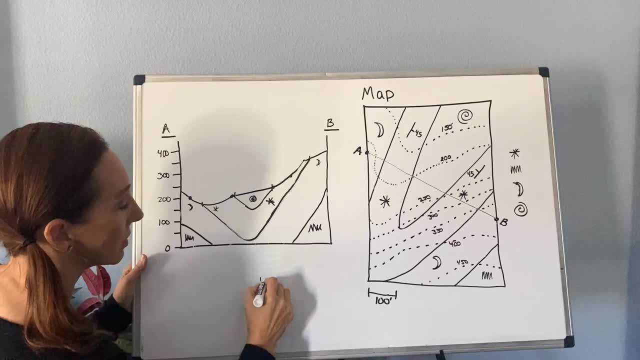 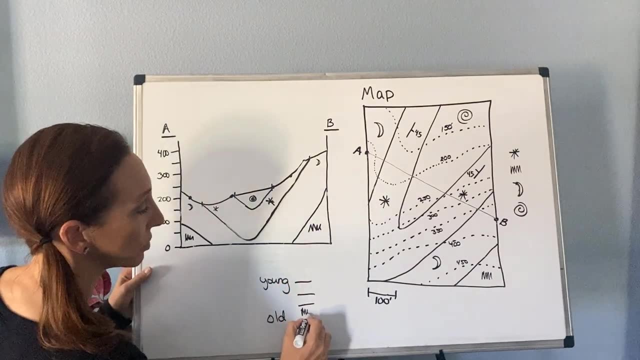 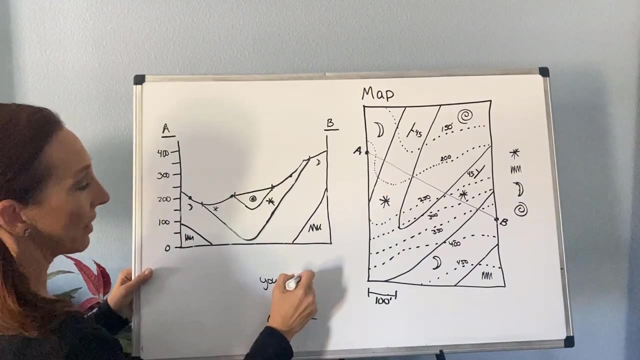 to youngest. so I would do old and then to young here. if I were to order those, my oldest would be my little squiggles, the next one up would be my little crescent moon, the next one up would be my asteroid and then the top one would be my little spiral. so different order than was presented over here. 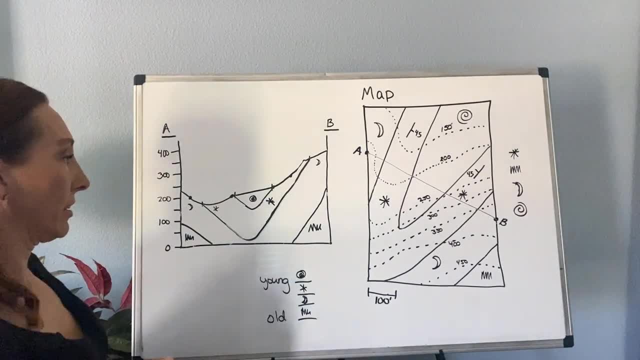 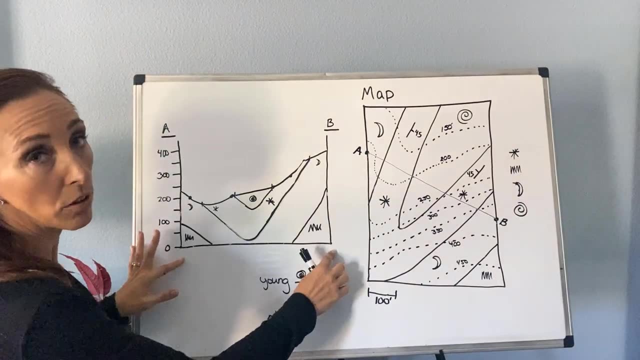 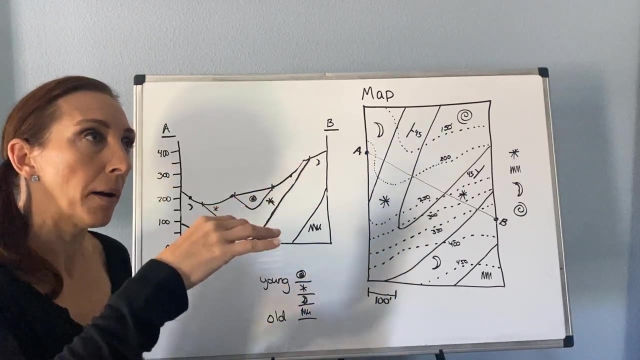 in the key, because now I actually know what was oldest to youngest. the last thing is um. sometimes we want to make sure that the vertical expression is the same as the horizontal expression on a cross-section, so that it reflects um, no, no vertical exaggeration, um, or a horizontal exaggeration, right? 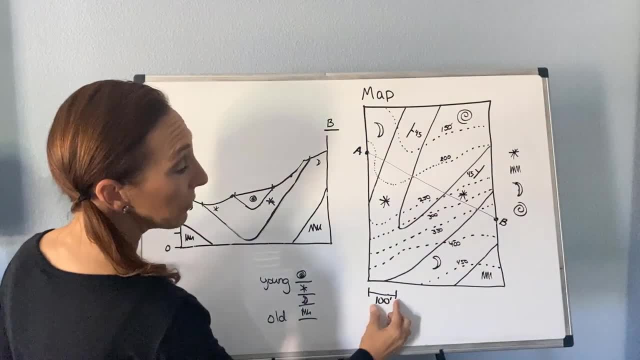 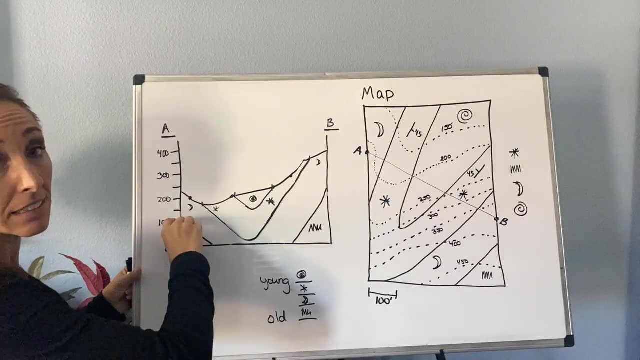 you want them to be the same, so to do that in this case- um, this is a hundred feet across my map, it's also a hundred feet across here- you would want to make the vertical axis the same, and you can see that the way I did that. it's approximately the same, so there is no vertical 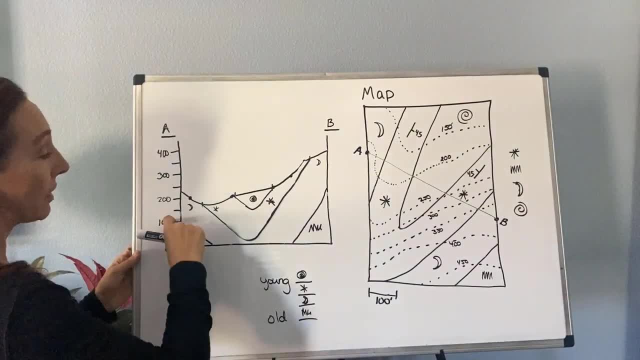 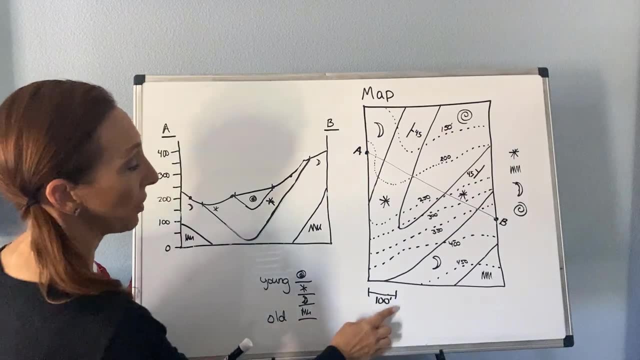 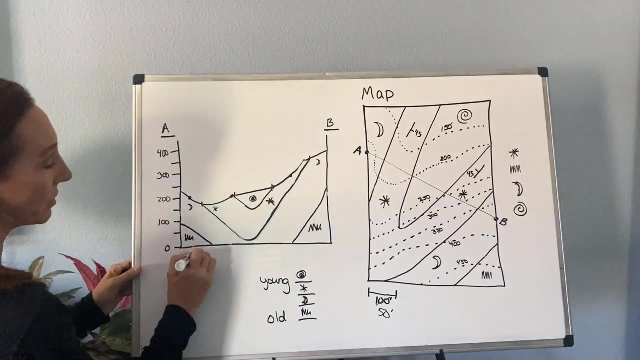 exaggeration here. it's just: a hundred feet laterally represents a hundred feet vertically. but let's say that if this value was different, if this value had been something like um 50 feet and so that now this is 50 feet, you would see that this is 50 feet laterally, but this is a hundred feet vertically, so you'd have a 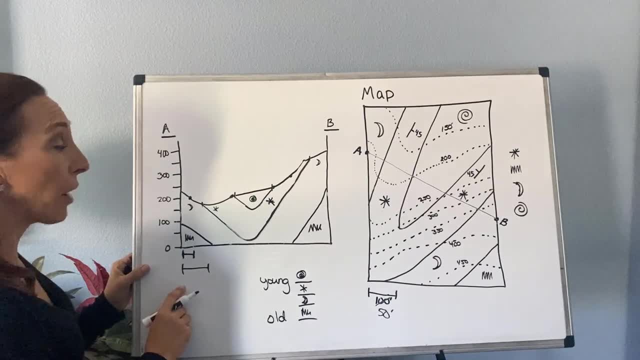 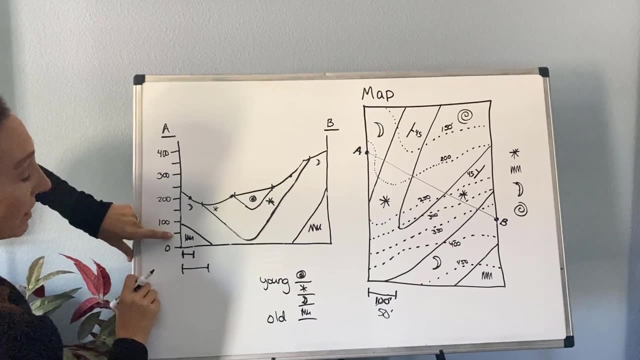 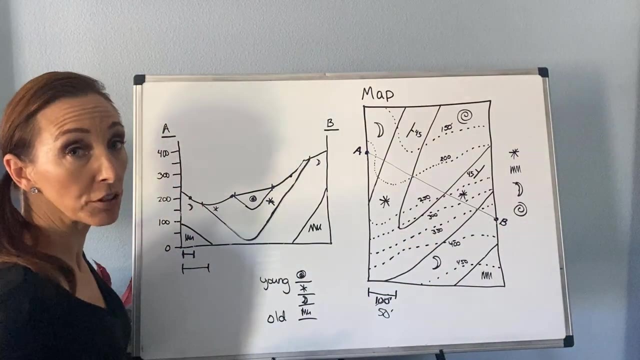 two times exaggeration there. if you wanted to fix that, what you would need to do is either compress this down, so each of these would be worth um instead of 50. it would be a hundred, uh, 200, 300. so you'd compress this down, or you would make your cross-section much wider to be able to make once.